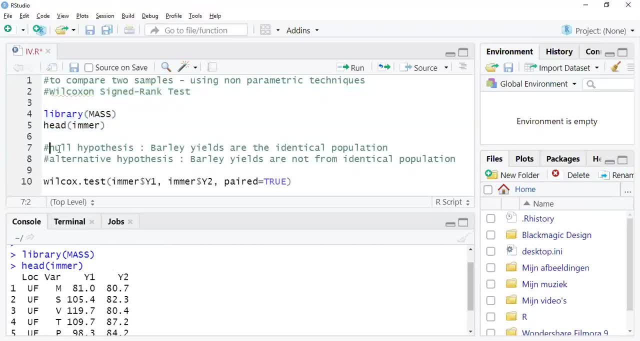 population. so null hypothesis in this case is that, uh, the crop rate and in this case barely, are both the eigen, are both from the identical population, and the alternative hypothesis is that the eles are not from identical population or they are from non-identical population. right? so there were two samples, y one and y two, and we will 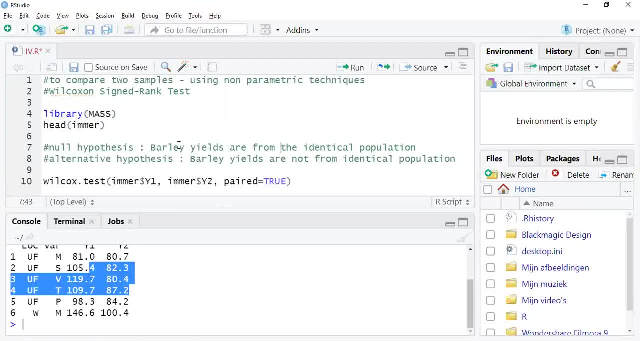 to compare non-parametrically using will cause the science sign drawing test. okay, so in r you have the wilcox dot test and then what you give as parameters is the two fields, right, the two samples, basically y1 and y2, and this is a priority test and we are doing here. we will see it at 95. 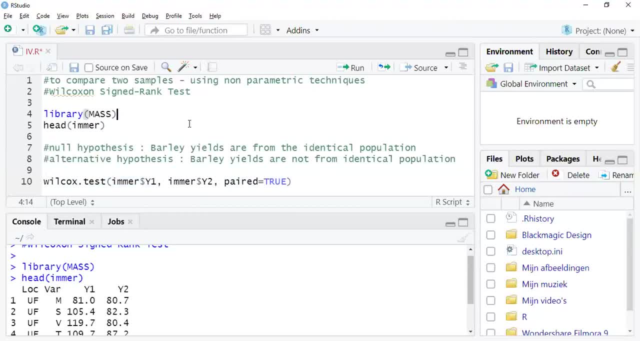 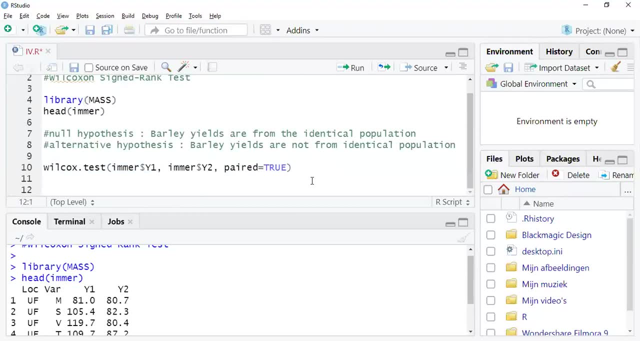 constituents level. so p value, uh, less than 0.05 or greater than 0.05 will decide the outcome of this test, and this is a parity test, so paired is equal to 2 and let's run this right. um, okay, fine, some warning message, but we have the results here and you will see that the p value is 0.005318. 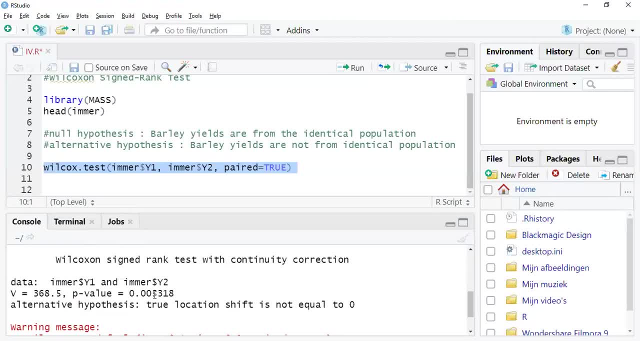 which is less than 0.05 right, less than the thresholds. so since it's less than the threshold, we will reject the null hypothesis. so null hypothesis is rejected and what we accept is alternative hypothesis. that means the crops are not from identical population. that's one way of comparing. you know two samples using non-parametric. 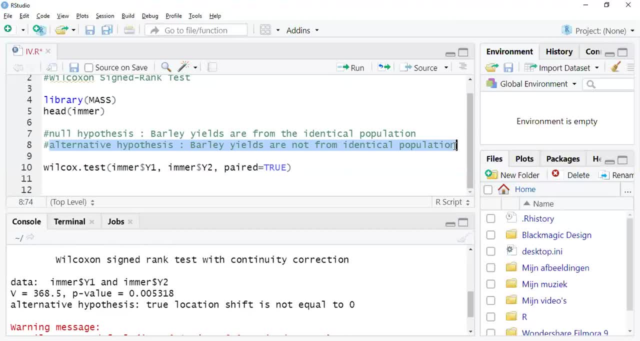 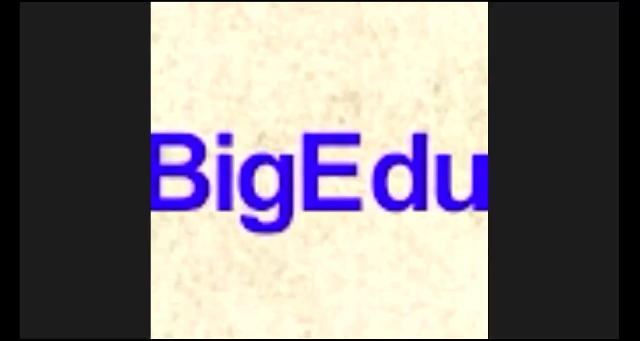 there are other ways also, and in another video i'll talk more about the other ways, but this is how you can compare two samples non-parametrically. thanks you.